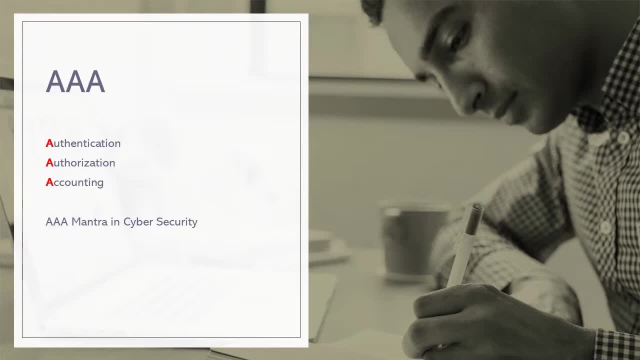 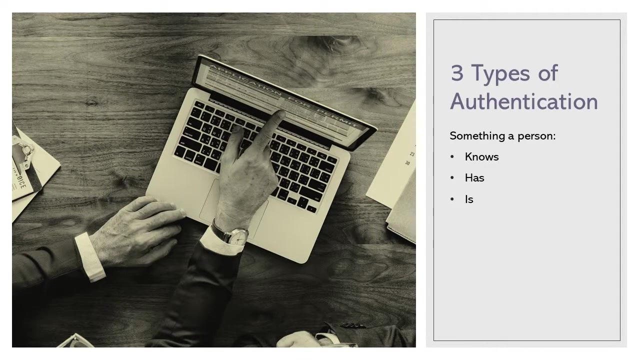 verified as being legitimate. The identity could be an ID, like a username, with the verification being a corresponding password, which together supports the verification. What are the three types of authentication? There are three types of authentication. These include something a person knows, something a person has and something a person is, Something a 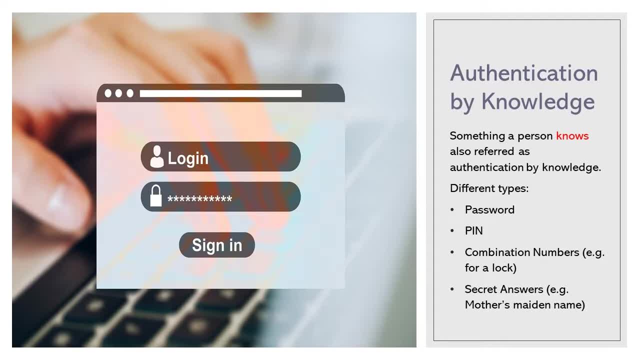 person knows is commonly referred to as authentication by knowledge. Different types of examples for something a person knows includes a password, a PIN combination numbers, example for a lock, secret answers- example: a mother's maiden name- To authenticate a person's identity. and. 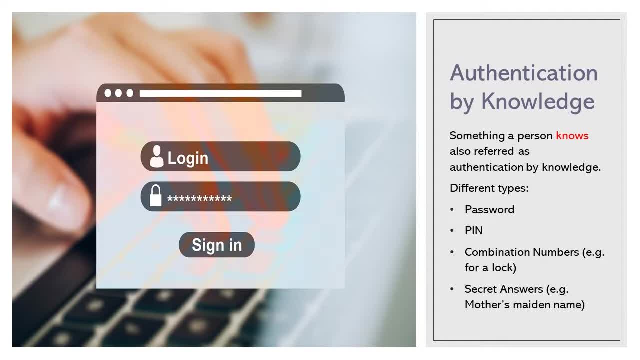 by something they know is easily achieved and is probably the least expensive method of authentication, but used alone, it doesn't really provide the securest methods of ensuring the identity involved is who they say they are, as the information involved, like passwords for example, could easily be hacked and used by someone else to impersonate the legitimate user. in an age where 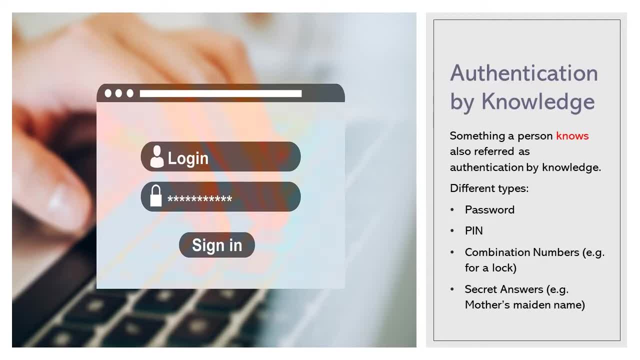 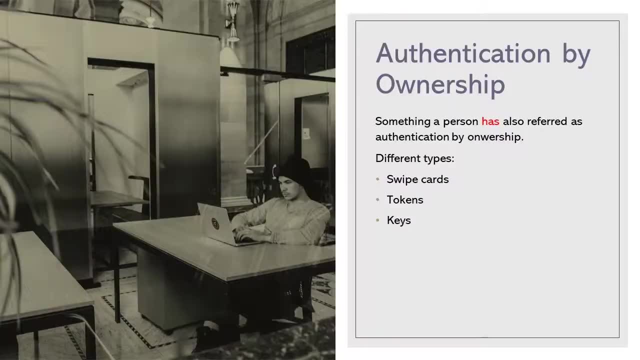 hacks and data breaches are commonplace, along with people using passwords, which, in themselves, can be easily guessed. a better form of authentication is required. something a person has is commonly referred to as authentication by ownership. different types of something a person has includes swipe cards, unique tokens, keys. the commonest example of something a person has is a. 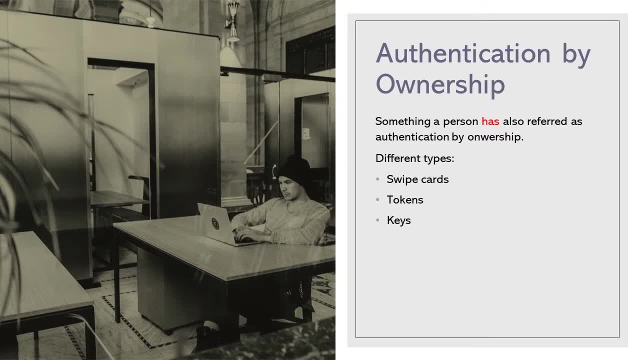 key. we all use keys in our lives to get, get into our homes, to open the doors to our cars, to start our car engines and so on. this piece of metal proves we have something that we can use to verify. we are allowed to access or use something. unique tokens are generated by little devices. 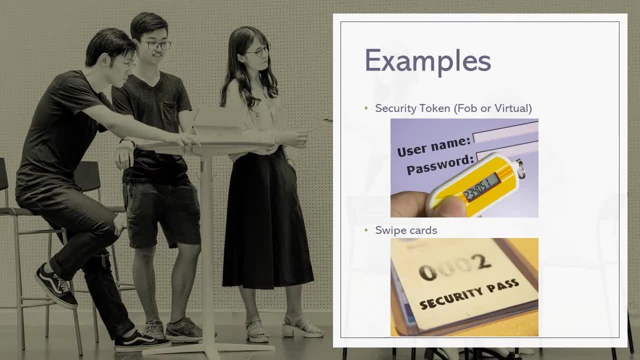 which cleverly use the current time and a reference seed number from a central source to work out a unique token for the person at that particular time. swipe cards can be used to make it easier to prove the identity of the card holder, so the person holding the access card can use it to swipe. 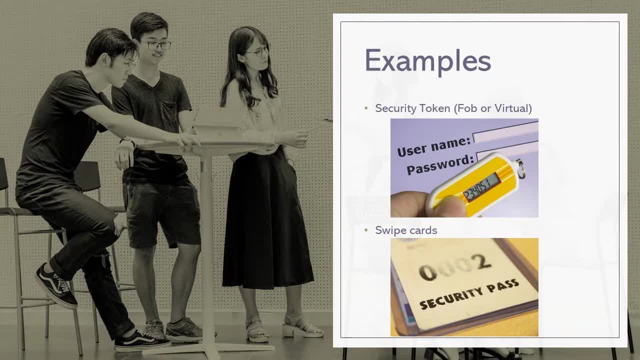 at an entry point like a barrier to get access, so the person holding the access card can use it to. they don't need to prove to security every time they want to access who they are, as the swipe card itself is sufficient to prove their identity. used alone, these methods of authentication won't. 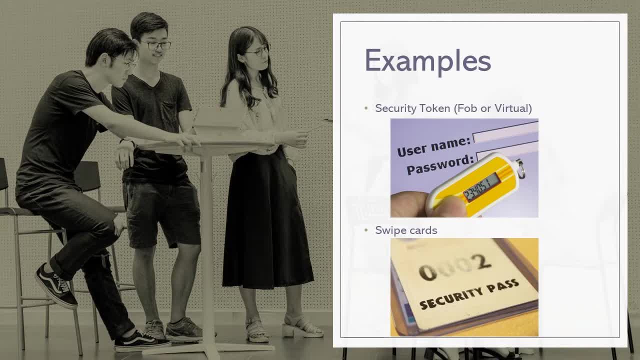 necessarily mean the person is legitimately without access, as they may not be the actual owner of these authentication items. they may have a set of stolen car keys or ones they've found. if the legitimate owner had lost them and armed with these keys, they can now open the car doors. 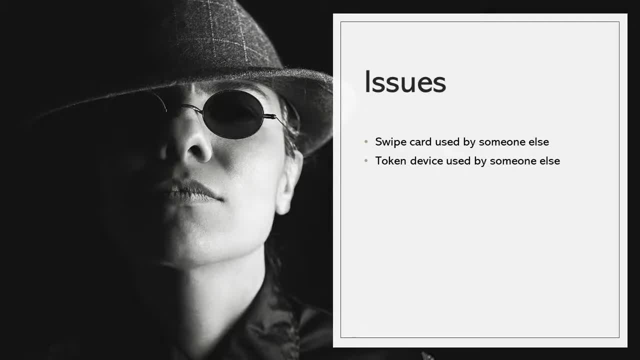 and get inside and start the engine using the key. likewise with access cards, most of these will have some form of chip inside with a reference to the person whose card it is, but if the card is in the wrong hands, the access card isn't smart enough to know this. so anyone who has a swipe card can use it to get. 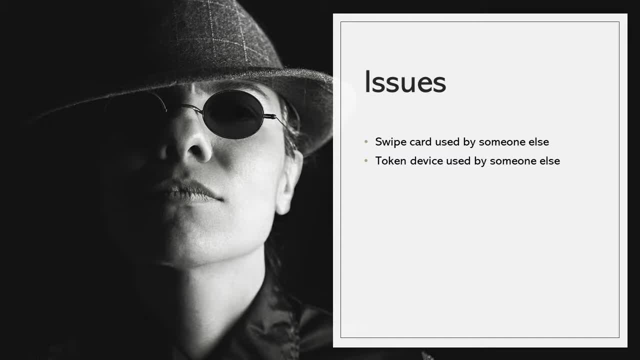 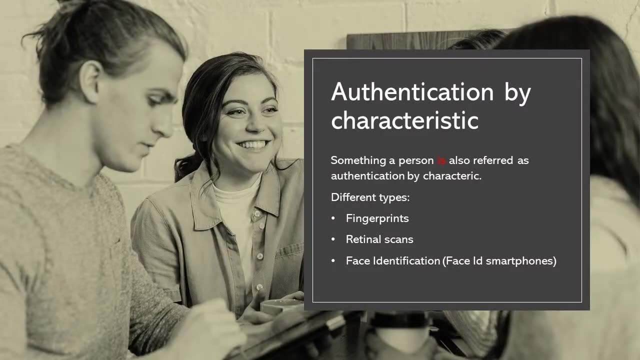 access, and so many people can be guilty of lending their swipe cards, especially when colleagues may have left theirs at home. the same holds true for the unique token devices, as, by having the token generated for the time it's valid means, access is granted. something a person is is commonly referred to. 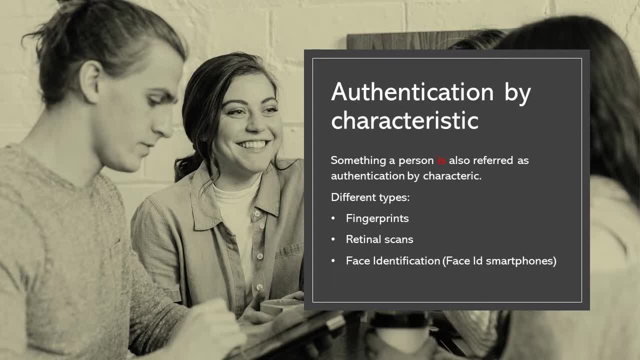 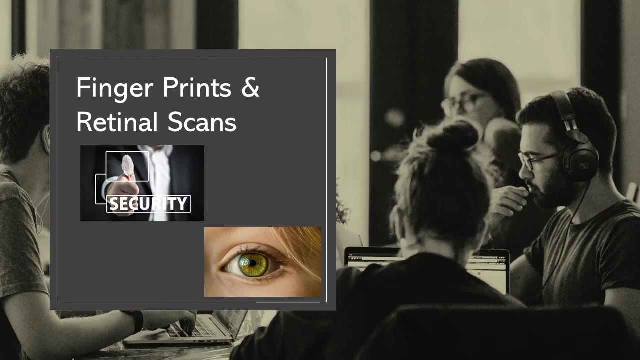 as authentication by characteristic. the characteristic is a physical characteristic which is unique to, unique to the person. different types of something a person is includes fingerprints, retinal scans, face identification, like Face ID on smartphones. fingerprints, retinal scans to Face identification- can be unique to individuals, so by using these, the identity of a person can be verified. This type of physical 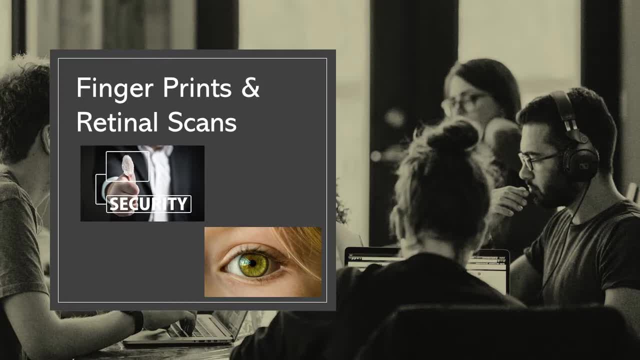 characteristic verification is known as biometrics. Many access systems these days use fingerprint access, from simple fingerprint access on smartphones to fingerprint readers to access secure locations. Whilst fingerprints and retinal scans are undeniably difficult to impersonate, checking them can be expensive, as the technology involved isn't necessarily cheap. so many 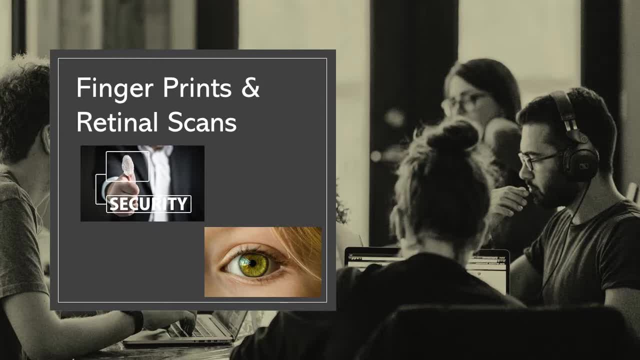 organizations simply won't use this form of authentication. The downside is the technology itself used for verification may not be foolproof. A Japanese cryptographer was able to create a fake finger using gelatin from sweets like gummy bears to fool fingerprint detectors. He was able to fool. 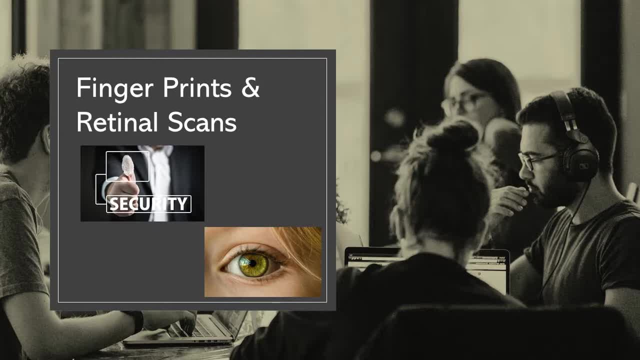 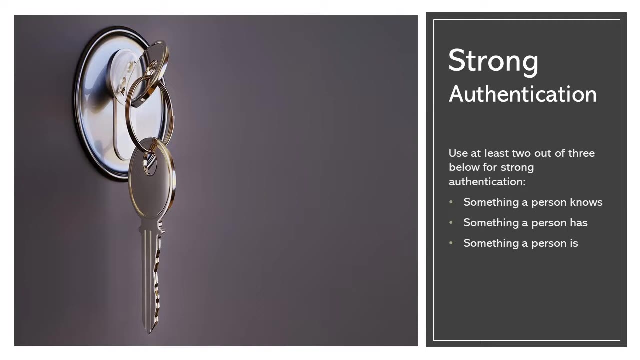 them four out of every five attempts, achieving an 80% success rate. The technology involved in checking biometrics is also expensive, so many organizations simply won't use this form of authentication. Strong authentication: To be able to perform strong authentication, at least two or all three. 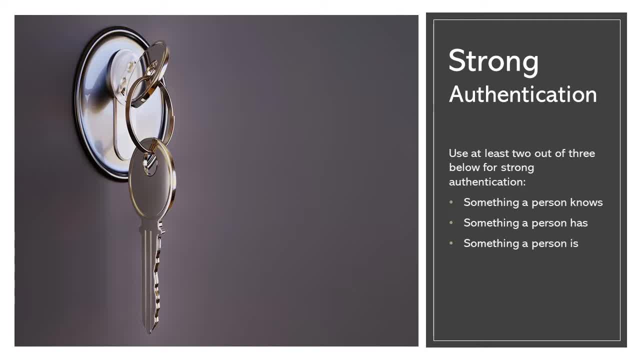 of the authentication methods of something a person knows, something a person has and something a person is, must be used. Each method of authentication alone only proves the identity of the person as far as they have the correct authentication item, be it a password, a swipe. 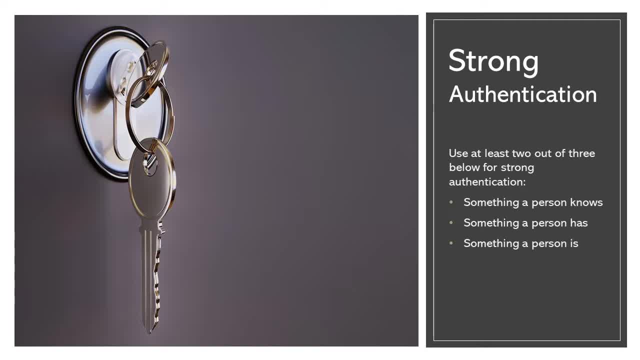 card to a fingerprint, But this may not actually belong to them and they may not be able to use it. A person may be trying to impersonate someone else, so any form of authentication to be strong, multiple factors must be used, so a person not only has to enter their password to prove. 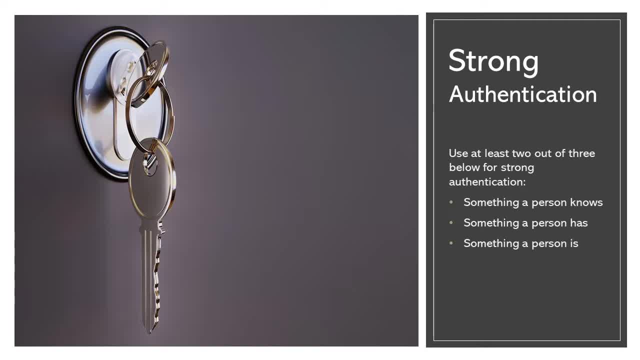 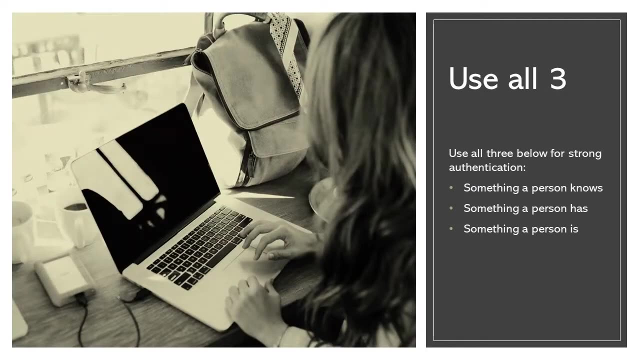 their identity, but they also have to enter the unique token on the smart code device that's assigned to them, thereby using something they know- the password- and something they have- the smart token- to provide a stronger case for authentication Are using all three methods where the person uses a swipe card that's assigned to them. 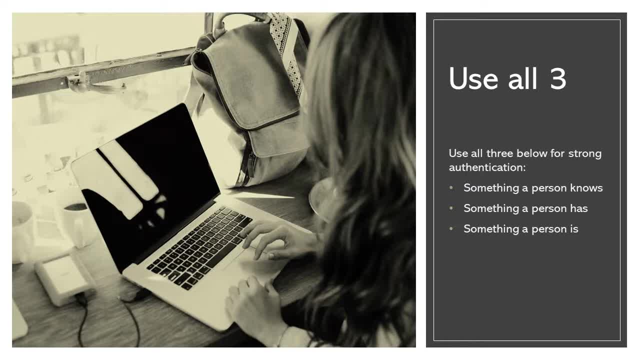 to enter an office building. they then use their password along with a fingerprint to log on to a computer system will make a case for strong authentication. So even if the swipe card was used by someone else, this person wouldn't be able to get access to the computer. 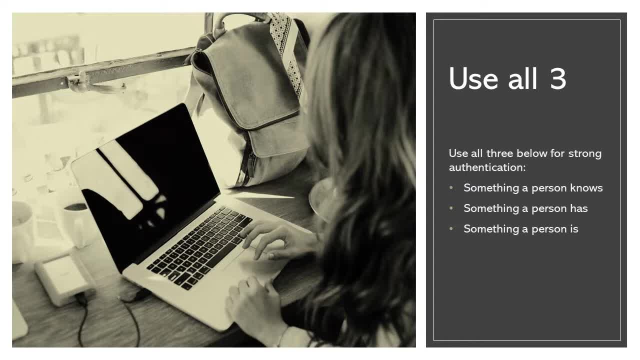 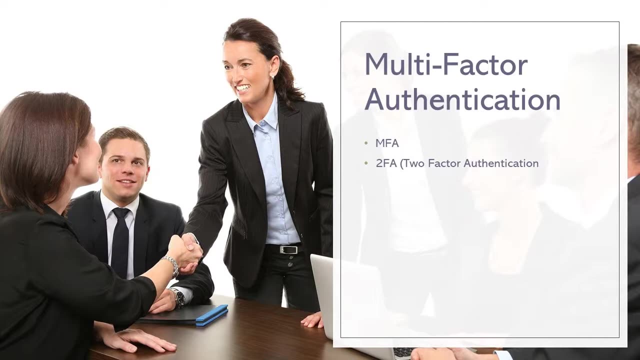 system because they were missing two additional forms of authentication: The password, known only to the correct person, and the fingerprint, a characteristic of the correct person. Strong authentication is also known as multi factor authentication- MFA for short- which means identity verification has taken place using two or more methods. 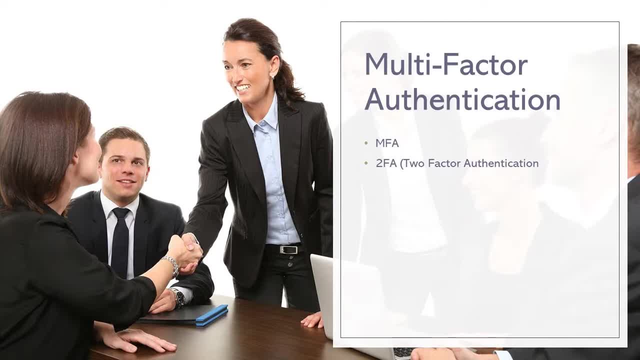 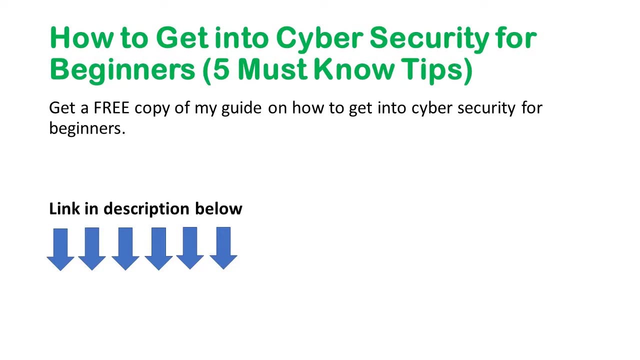 of authentication When two methods of authentication are used, the term two factor authentication, 2FA, is commonly used instead of MFA, even though it's still a form of multi factor authentication. Thanks for viewing this video. Don't forget I have a free guide called how to get into. 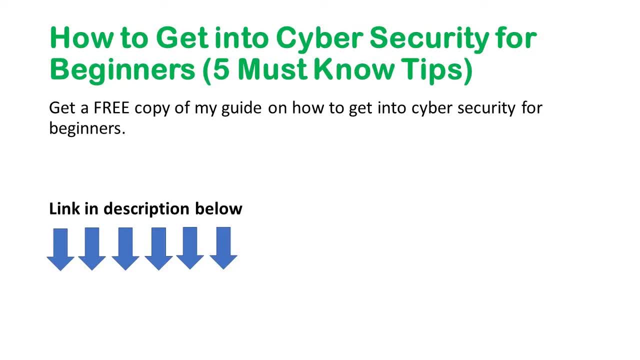 cyber security for beginners, where I showcase my five must know tips for anyone considering a career in cyber security. The link is in the description below. Till the next time.